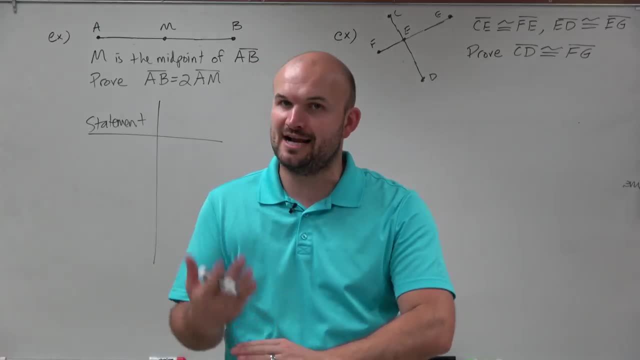 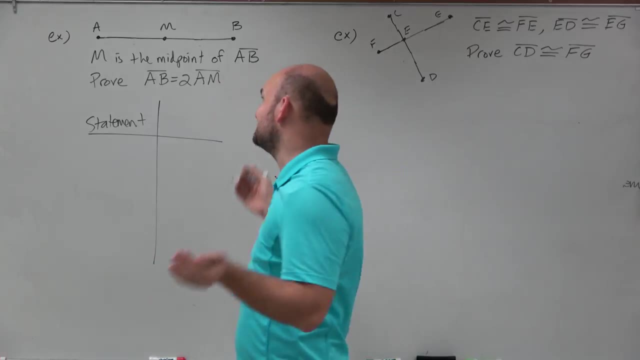 We've got to provide step-by-step justifications that order us to come to that conclusion. We just can't say: well, I know it's true, and that's QED, It's all done. So we're going to have a statement and then a reason. 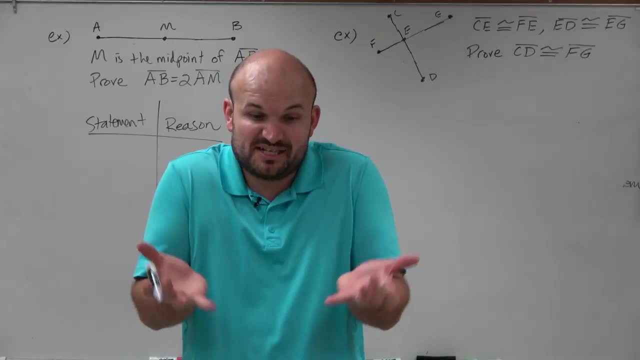 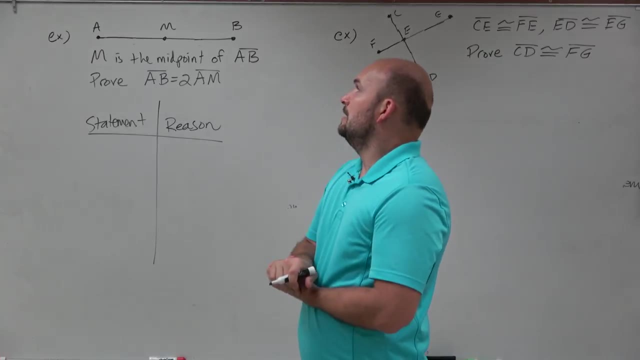 So the first and easiest statement to always do is start with what you know. Get your building blocks. What is everything you're given? So in this example, we have a figure And we don't need to write that we have a length. A, B is cyclical. 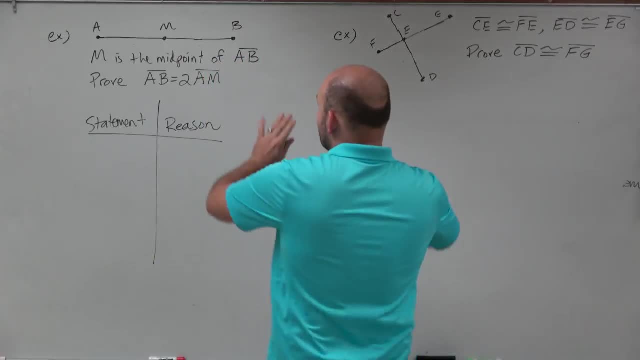 You know that's given, But let's write down some of the information that we're given And you can see from this point they give us that M is the midpoint of A- B, So that is a great thing to write down as a given. 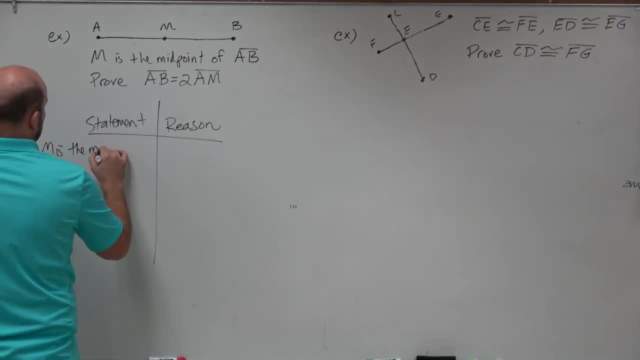 So I'm just going to write: M is the midpoint of A- B. Okay, And why do we know that M is the midpoint of A- B? Because it is given. So we're just going to write given Now they wouldn't tell you that M is the midpoint. 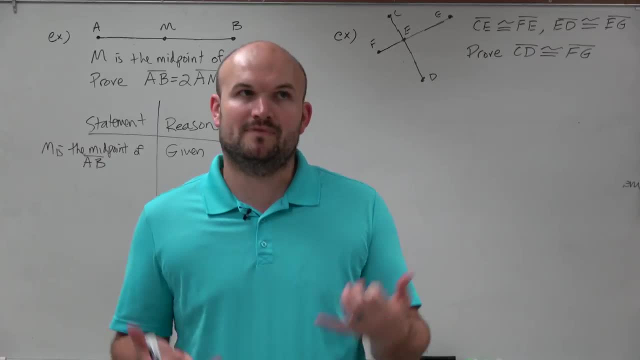 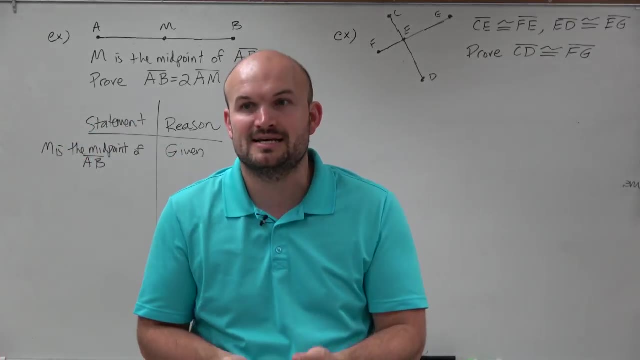 Unless they wanted you to use the definition of midpoint somehow, Or the fact that we have a midpoint somehow. So we have to think: you know what does the midpoint mean? Why would they tell us about the midpoint And how could we use that to prove to you know? help us use that in our proof. 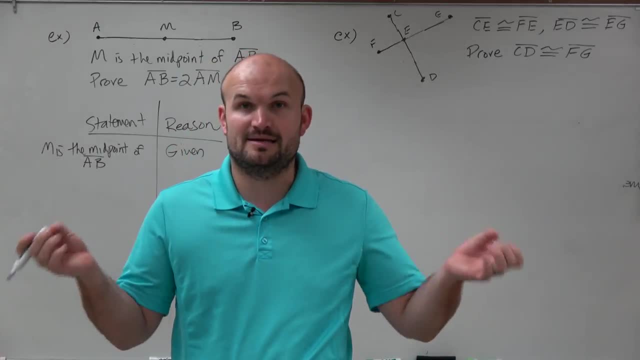 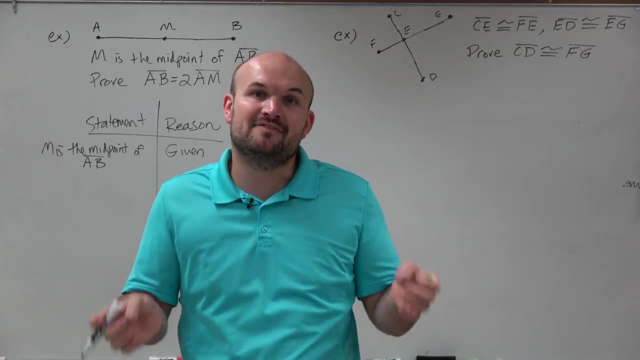 Well, the main thing of the midpoint, remember, a midpoint is basically a point that's in between two other points, And if those two points are on a line, then that midpoint, kind of you know, bisects that line, Basically cuts that line in half. 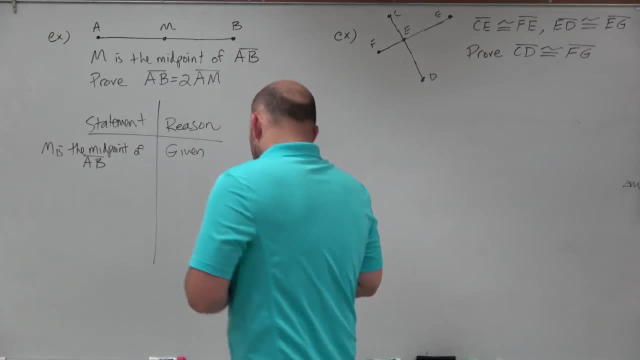 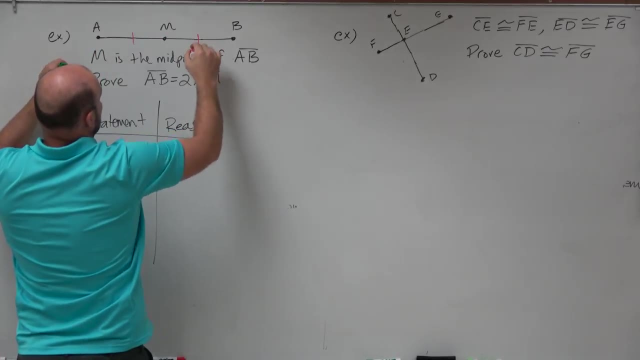 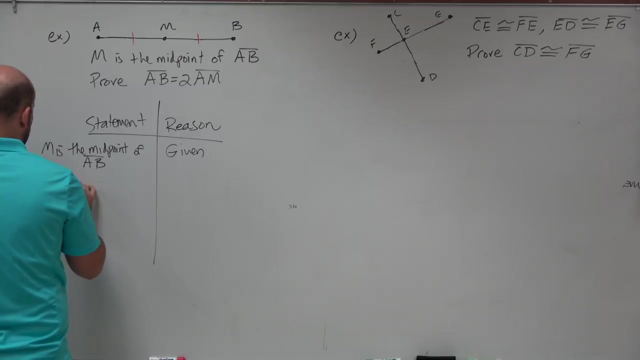 So, therefore, both two segments are now going to be equal. So we have this nice long segment here. A- B, Since M is the midpoint, that now makes both those two segments congruent, Equal in measure. So now what I can say is A- M is equal to the length of M- B. 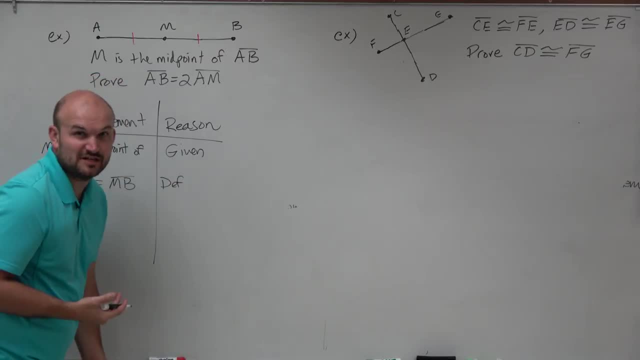 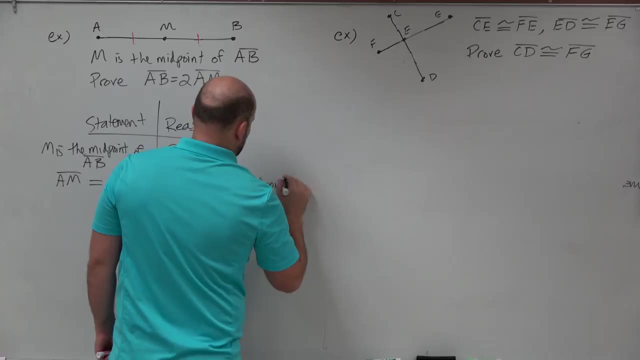 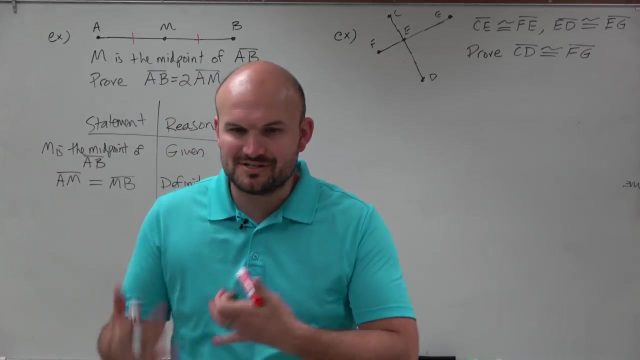 And that is because that's the definition. A lot of times we can just write definition as D, F, But I'll write the whole thing out. Definition of midpoint. Okay, So we have the definition of the midpoint. Now the next thing is: you know what else can we do? 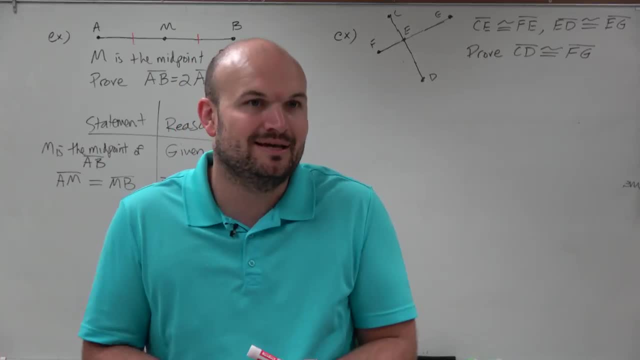 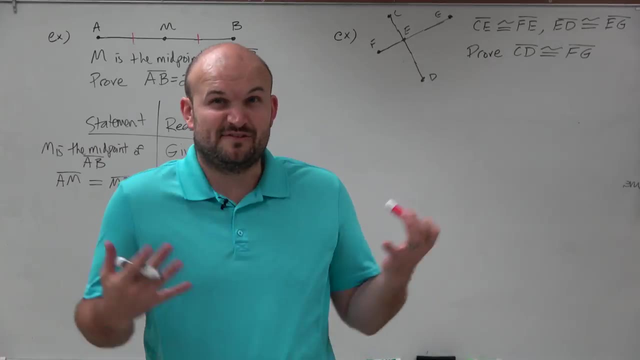 Now, I started off by saying we're going to use the segment addition theorem And that's going to be kind of the highlight of what we'll be doing here. You know, sometimes you might be using it, Sometimes you might not, But I think it's a good way to start. 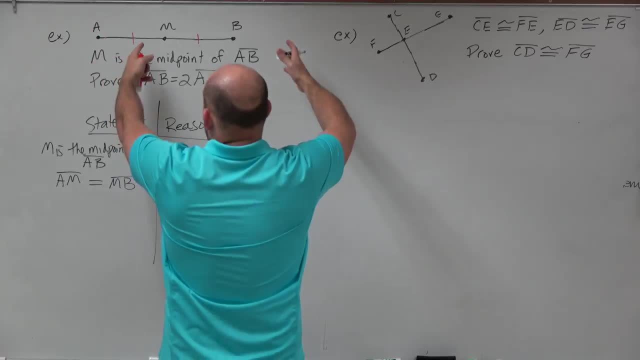 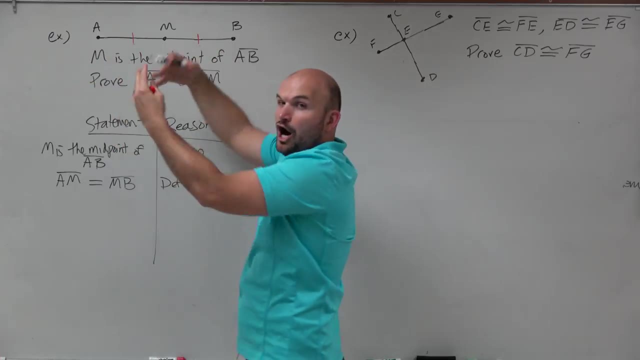 If you're kind of stuck. well, we know that whenever you have a segment, if you have a point that breaks up that segment, the sum of the two parts that you broke your segment up to are always going to add up. So that's going to be the definition of the midpoint. 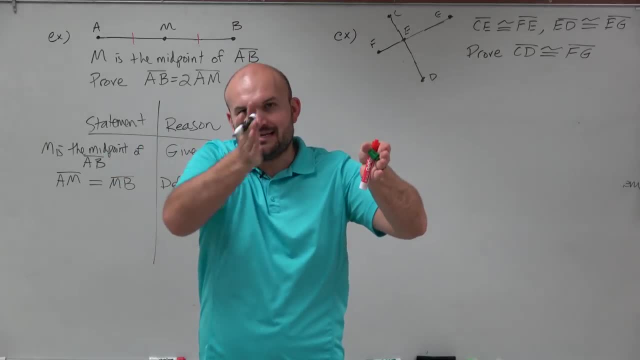 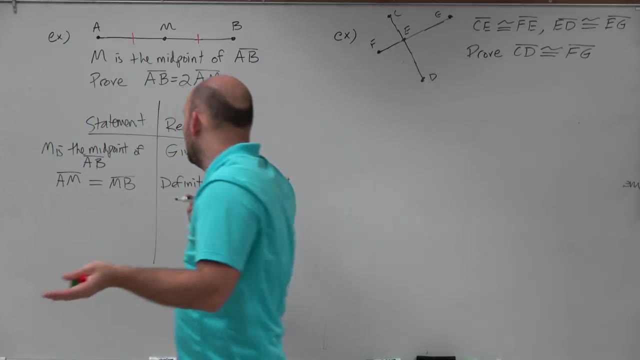 It doesn't matter. you know, if I take a segment, it doesn't matter how many times I cut it up, the sum of all those little parts is still going to equal my whole segment, And that's basically what the segment addition theorem states. 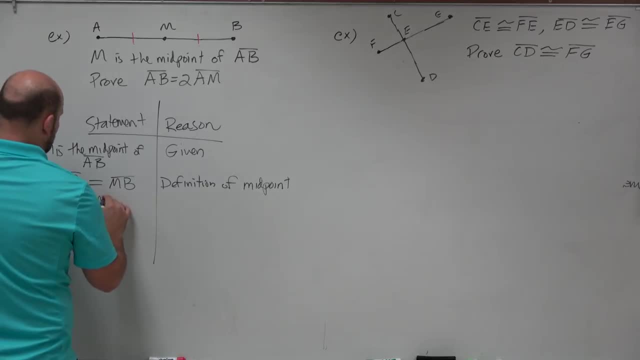 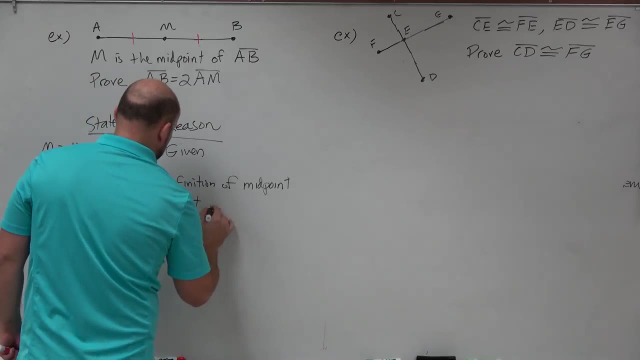 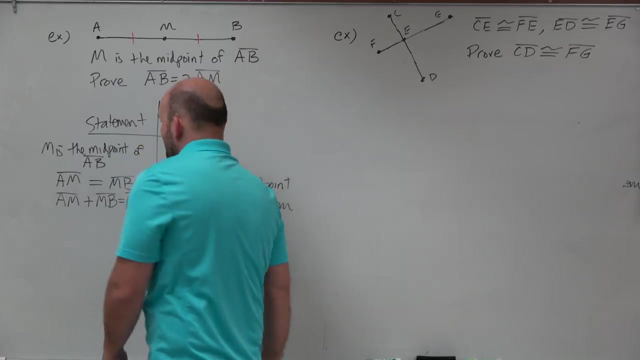 So I can write: AM plus MB is equal to AB, And that is my segment addition theorem. Okay, So now, Now we have all this information, We've written down basically everything we know, as well as everything that we can think of. that would be important. 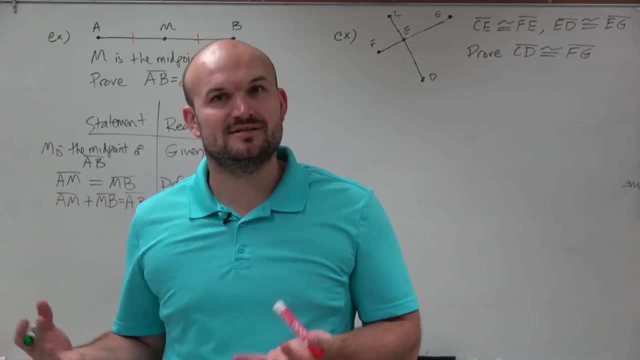 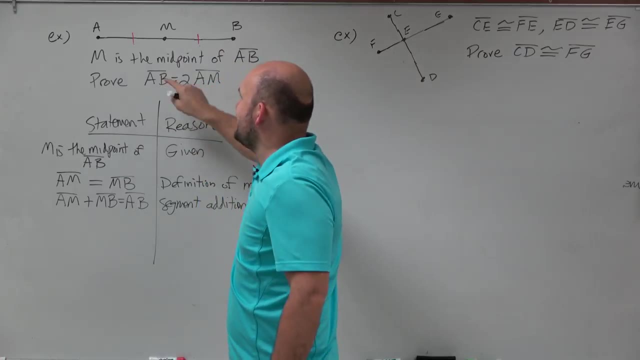 Here comes the trick, the tricky part. How do we take all this information now and then write it into a justification? you know a meaning that we can say that proves AB is equal to 2 times AM. Okay, So what? that comes up with the kind of tricky part. 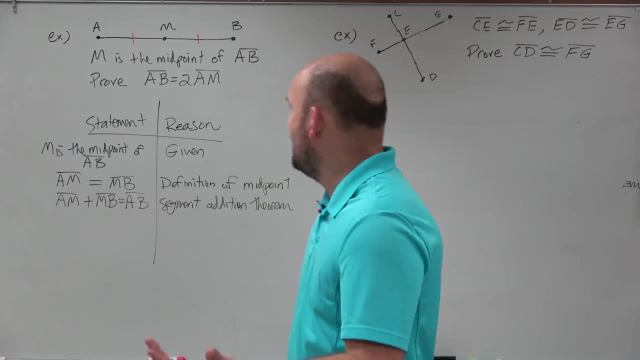 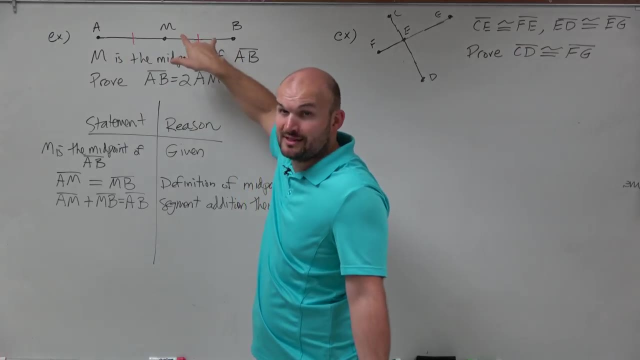 and it's going to happen over and over, and that's why we want to get practice in this. you to look at it, You know, think about this. We're trying to get 2 AMs. We know that AM and MB are congruent, right. 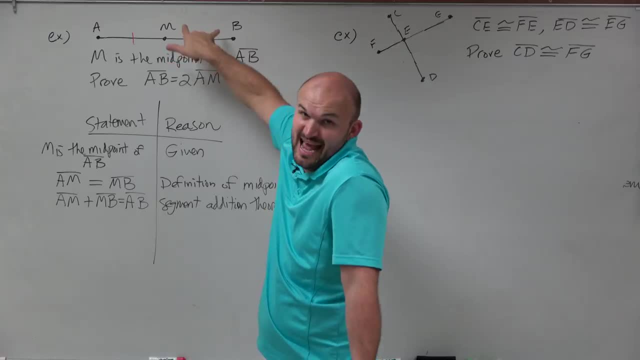 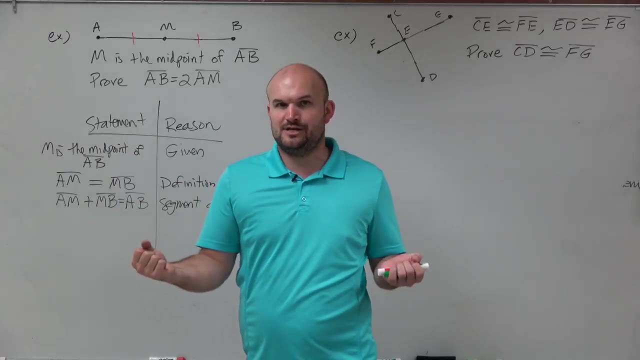 They're equal in measure, And so we could say that that's AM and that's technically AM as well, right? So AM is equal to MB, which we said there. So if they're equal to each other, then it doesn't matter which one I use, right? 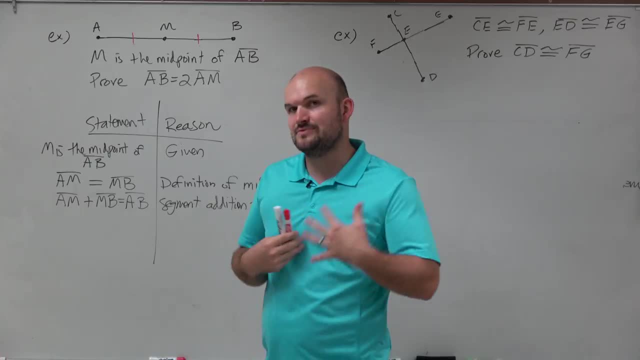 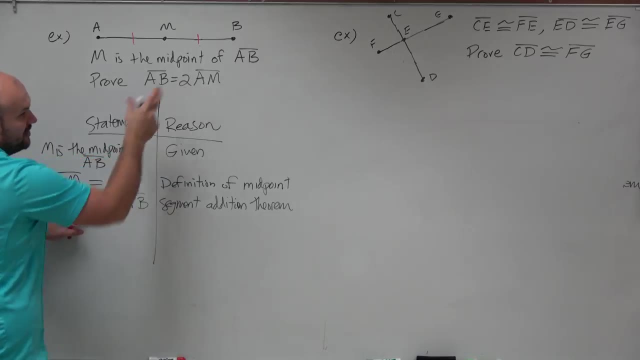 I could substitute one for the other, And that's what we're going to use for this. next step is substitution, Rather than writing MB. there's no MB in my proof right. You always want to look at what you're in. What are you trying to prove? 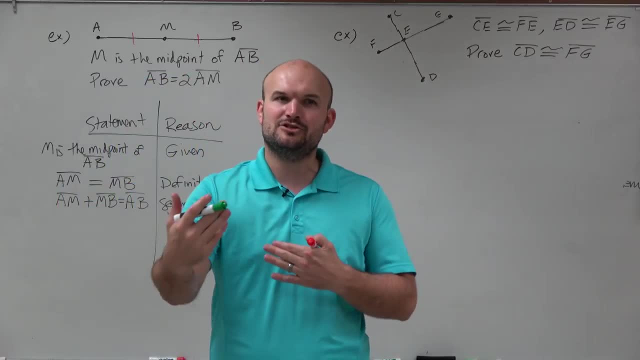 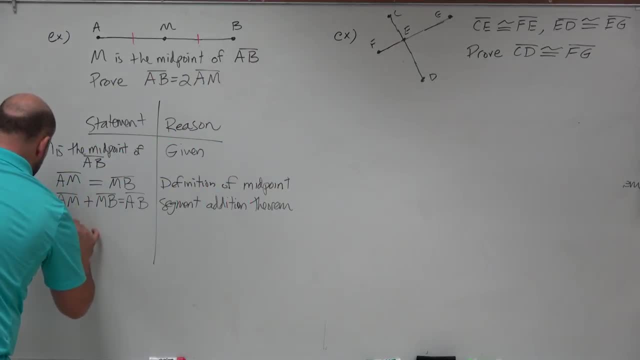 to help you with your proof. So what I can do is say AM plus AM. I don't need to write MB, because MB is equal to AM. So AM plus AM is equal to AB. Why? Because I used substitution. I substituted in the length of MB in for AM. 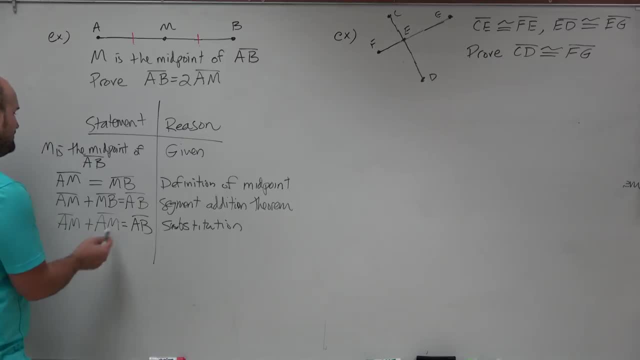 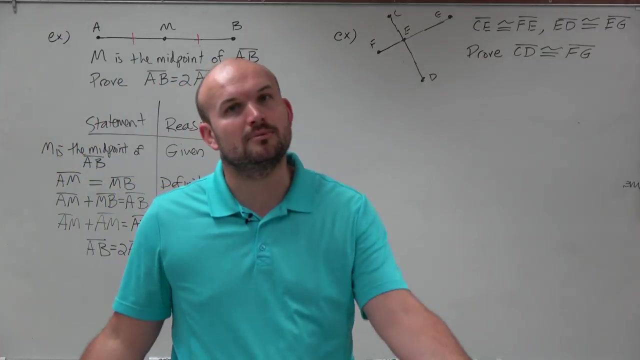 Now I have AM plus AM, which is going to be 2 AM. So I can just write: AB is equal to 2 AM, right? And then the reason. therefore, I can just write: simplify, OK, And then we can just use my box to say my end proof, my proof is complete. 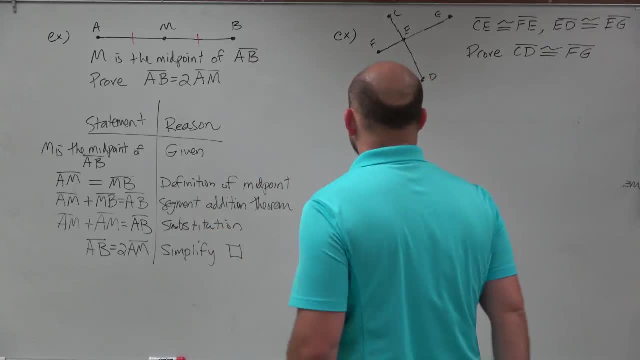 OK, You can also read, write the other way and then switch it around if you want to go through. So you can just write, write the other way and then switch it around if you want to go through. So you can just write, write the other way and then switch it around if you want to go through. 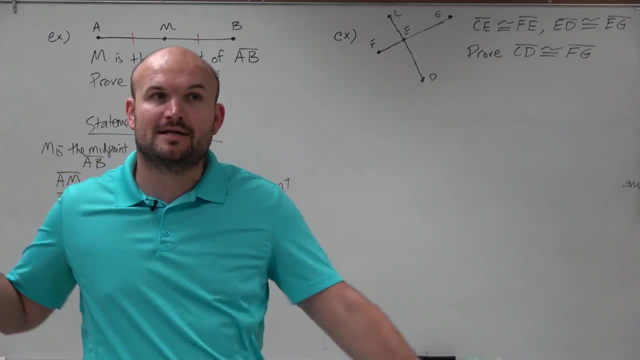 OK, So in the next one, next example, we have a two-count proof, So we automatically know: well, let's just get our statement and reason. We know that's what we're going to be using, So let's write the statement and reason. 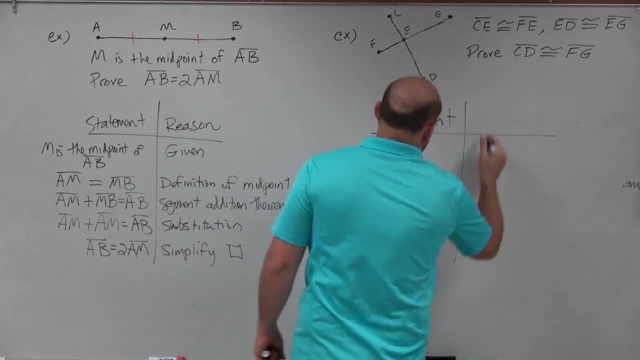 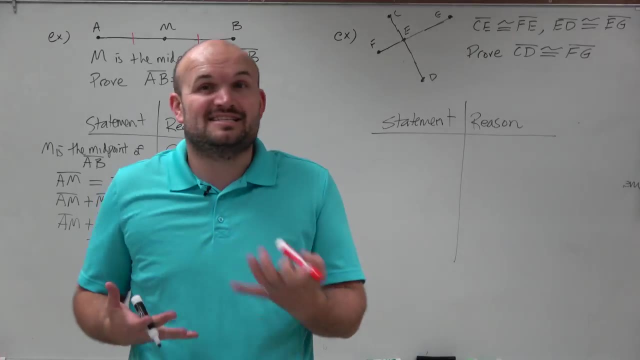 And a lot of times I get with students and they're having trouble with proofs, which I think many people can feel your pain in going through it And one of the ways is to just be like: well, I'm just going to get started with this. 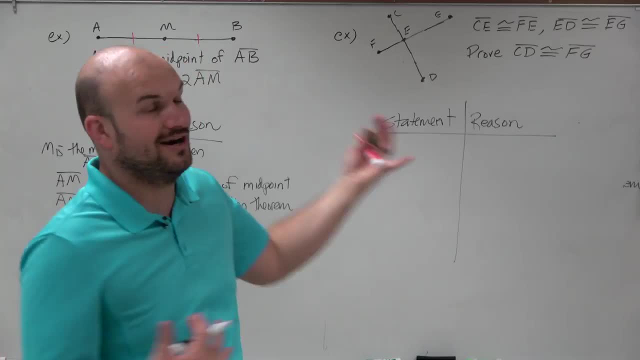 I know I'm going to use a two-count proof And let's just go and get started with writing down what I'm given. I might not even know what all this stuff means, But I'm just going to write it down in my proof. 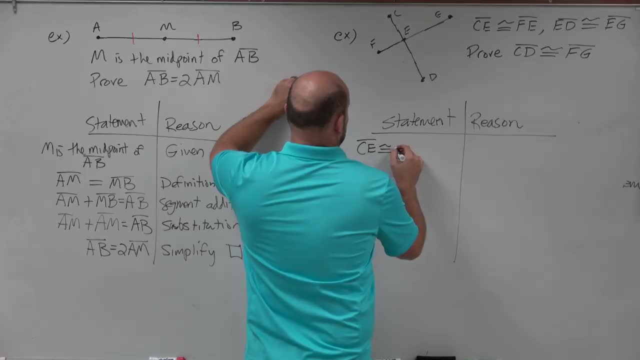 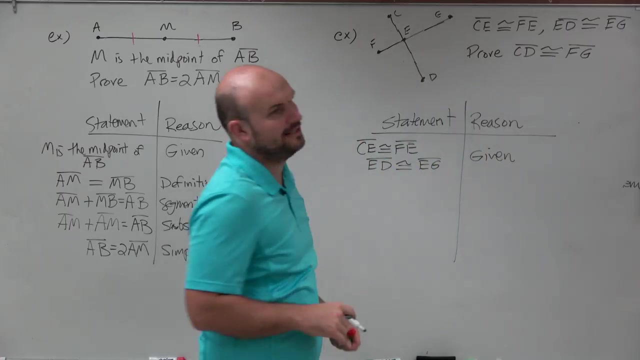 So I'm going to say that line CE is congruent to line FE- I don't know why I keep on doing that. And I could say ED is congruent to EG. And why is all that true? Because it's given. So now, once I wrote it down there, let's actually see. 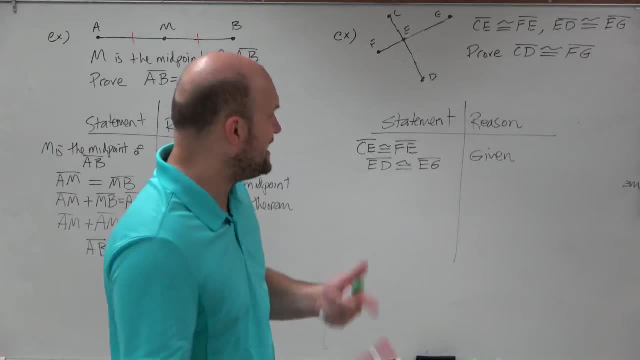 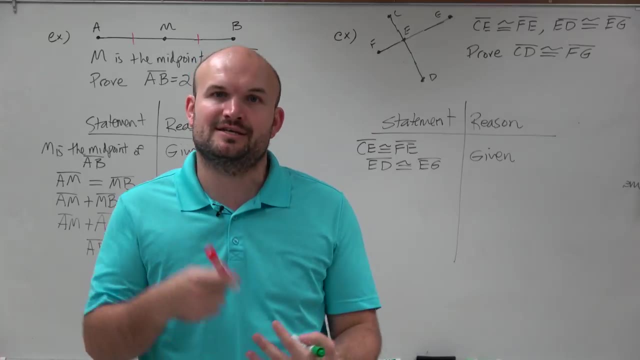 how is this actually going to make sense? How is this going to help me? And writing this stuff down is great. Possibly it might give you some partial credit on a test or homework, But to me it's helpful to visualize everything, So I always like to. if it's in a book, I like to redraw the figure. 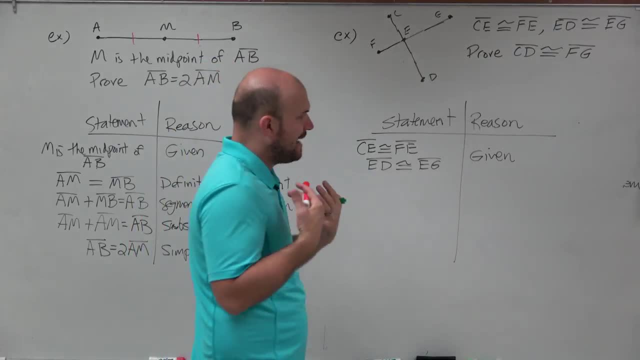 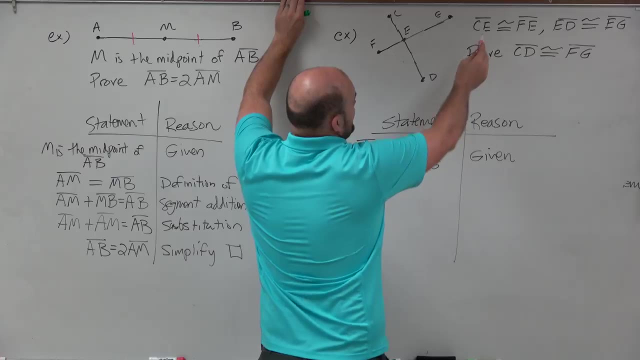 So therefore, I can write it and visually see what is going on. So when we have segments that are congruent, that means they're equal in measure. So I'm going to use tick marks to show that they're congruent. So it says CE is equal to FE. 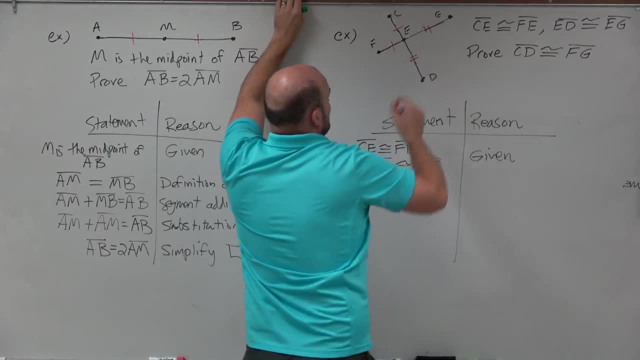 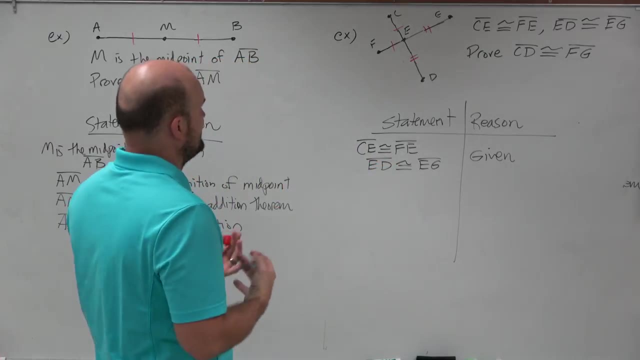 And then ED is equal to EG. So how can we use this information now to our basic advantage? How can we simulate a lot of this information? Well, one thing that I kind of notice here is- I know that again I've taken a segment- 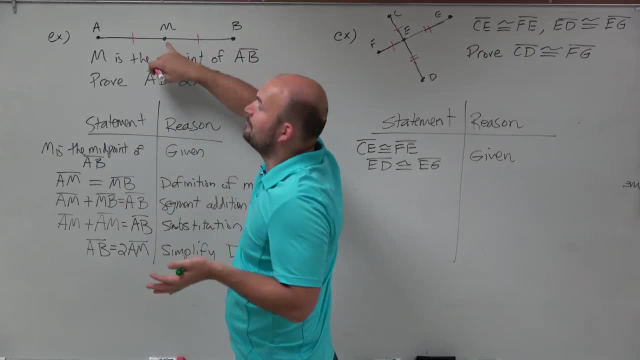 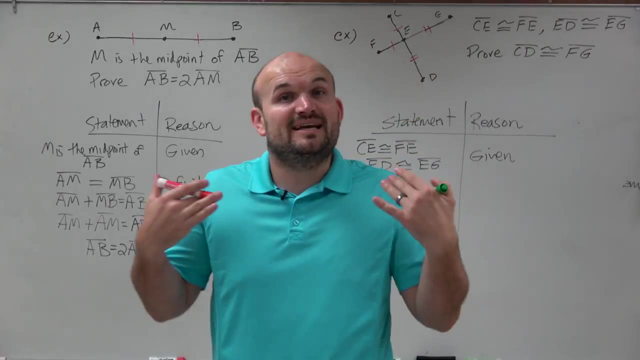 and I've broken it apart. Over here we took a segment and we broke it up by using the midpoint. Well, here we're taking a segment and we're breaking it up by using an intersecting line, So therefore we can use the segment addition theorem. 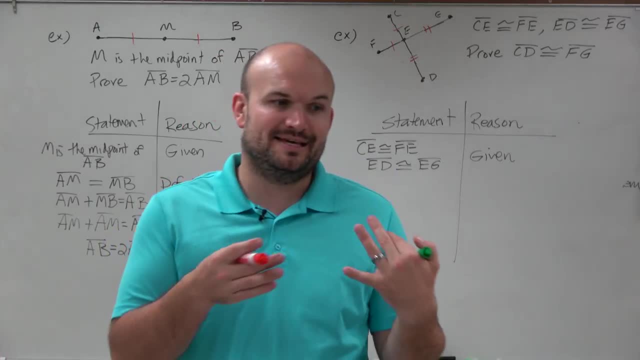 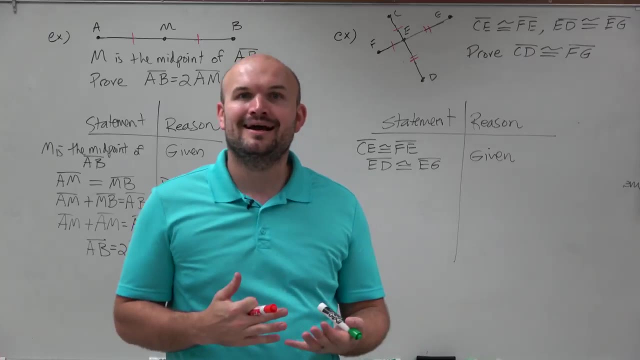 Again, I don't know if that's going to help us or not. Obviously, by the title of this video you know that it is going to help us, But when you're thinking of a problem that you don't have really any information for, 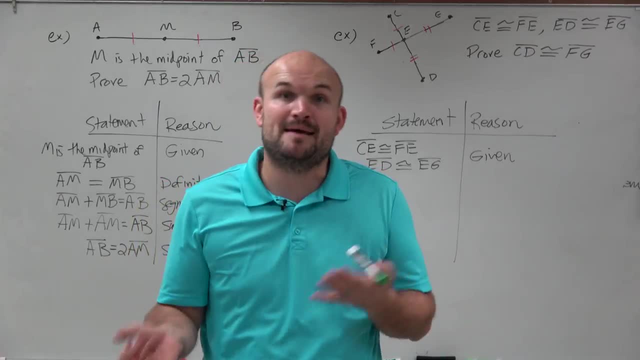 if you know that you have a segment that's being broken up, well, hey, you can write it down. Maybe it will help you. Maybe it won't, But you've got to at least try. Try to see if it can help you out. 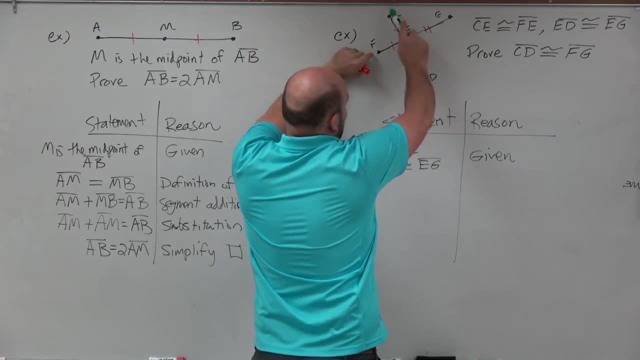 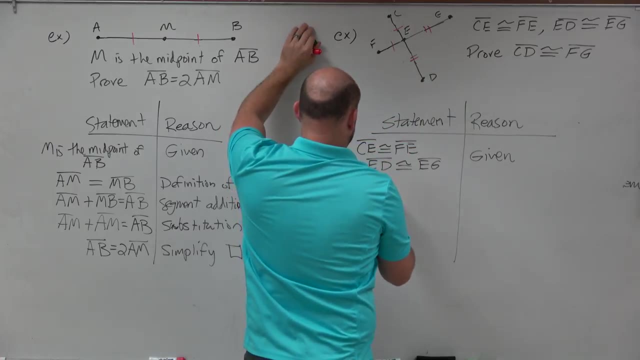 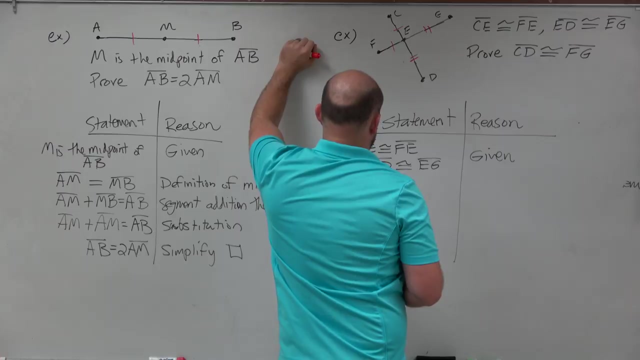 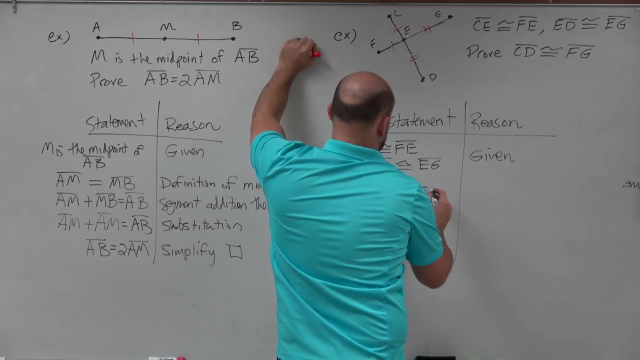 So let's go ahead and write a segment addition here. If I have this length CD, you could see that CD is being broken up by CE and ED. So I can say that the line CE plus CE is length of CE, is plus the length of ED is equal to the length of CD. 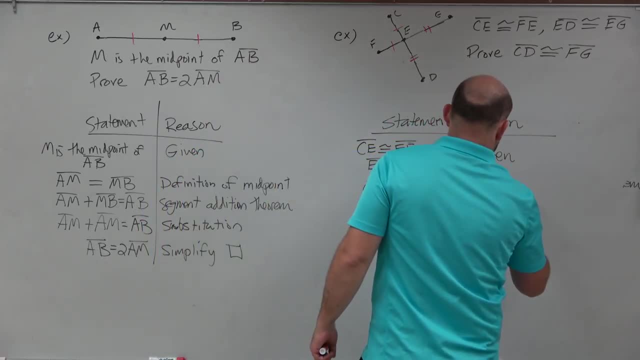 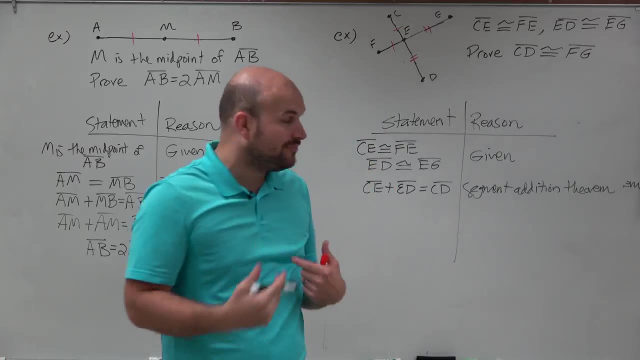 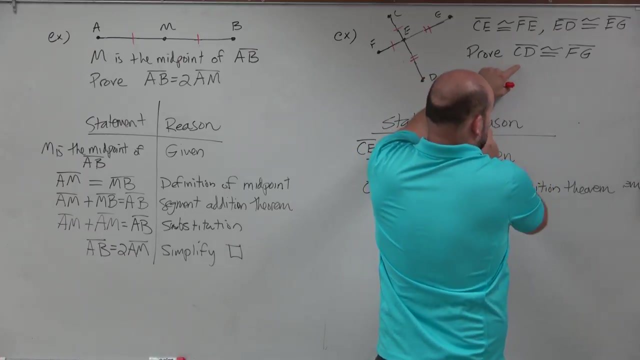 And that is going to be your segment addition. Now, what's important, though, is, again, remember going back to that substitution rule Again. the end is, we want to prove that CD is equal to FG, So one thing I can do: 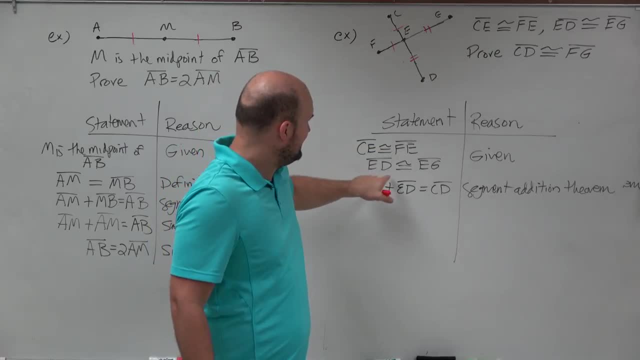 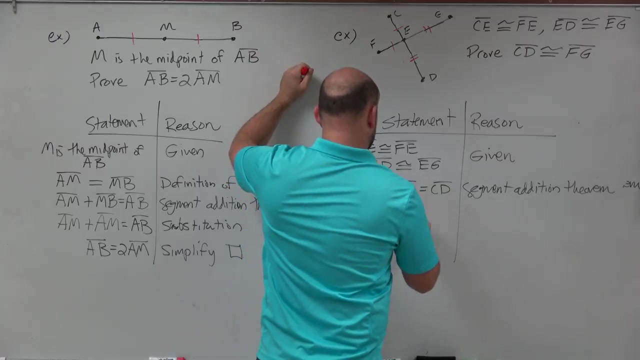 What I can do is, well, CE is equal to FE And ED is equal to EG, And FE and EG are equal to FG. So I don't know. Let's just try substituting this and see what happens. So I could also say that ED plus EG is also equal to CD.